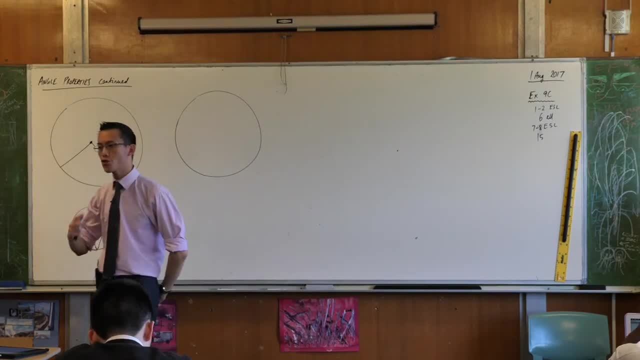 angle at the center here. But if I don't draw the angle on the circumference at a nice neat spot, like up here, if I draw it at an awkward spot, like say over here, the diagram you get looks quite different. This is what it looks. 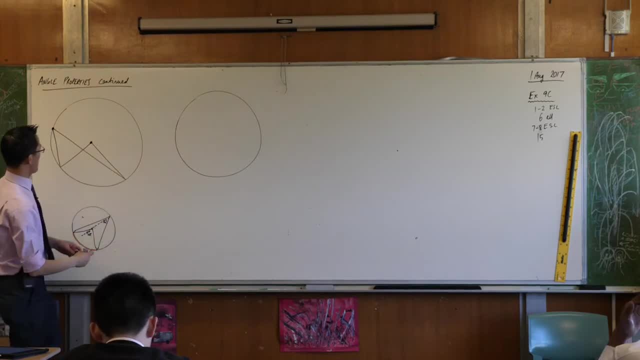 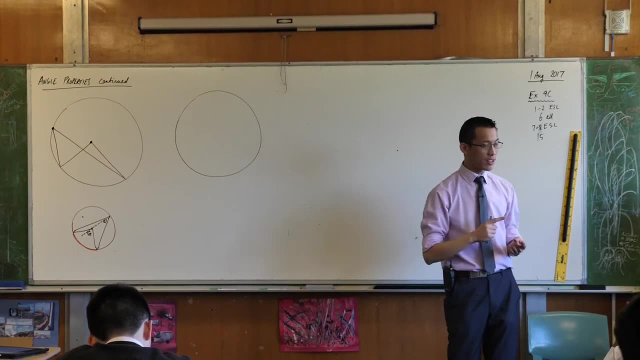 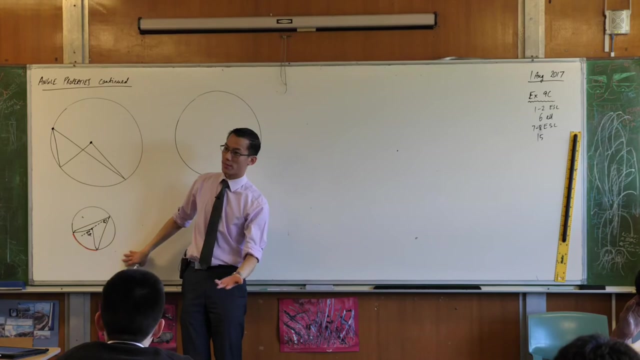 like: Not bad, This is the same situation: Angle at the center, angle at the circumference, standing on the same arc. In fact, the property still holds, which is one of the lovely things about it. However, I can't like. 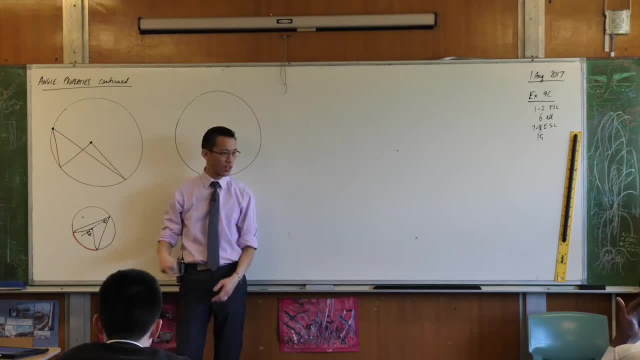 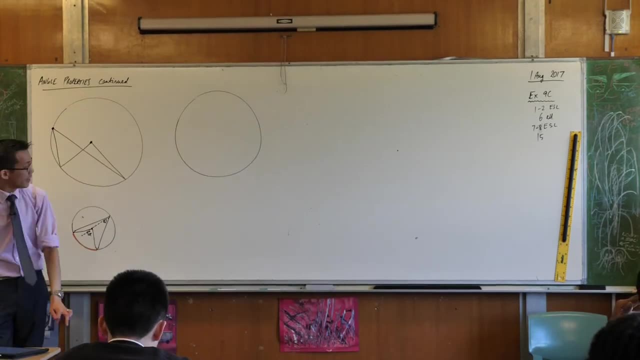 where would that line go? See my line that goes through the center. It's not going to divide that thing up in two like it did before nice, and neatly. So how is this going to work? Interestingly, it is still going to work, remarkably simply. So remember this time. 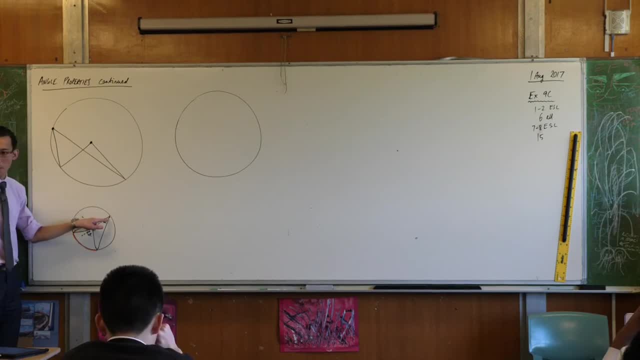 last time, rather, I drew a line from the point of the circumference to the center. I drew that radius. I went a little bit further so I could do that exterior angle of a triangle thing. I'm going to do the same thing over here. So here's the angle at the circumference. 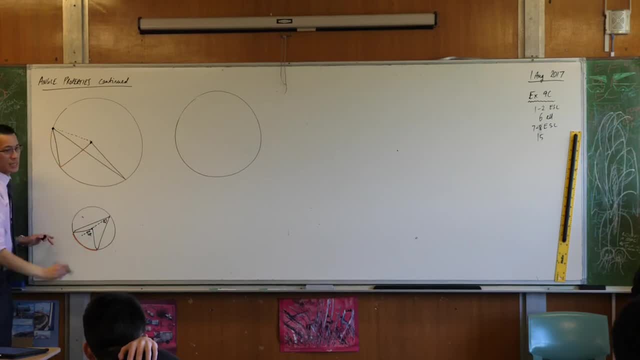 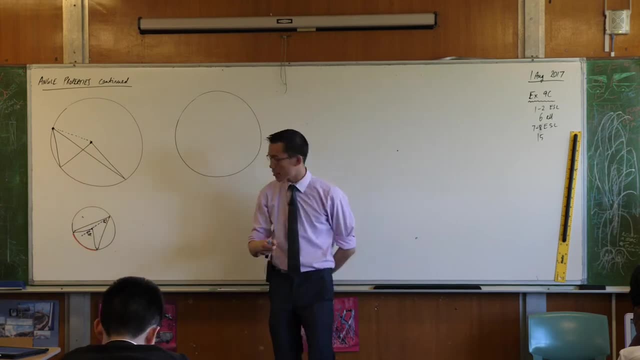 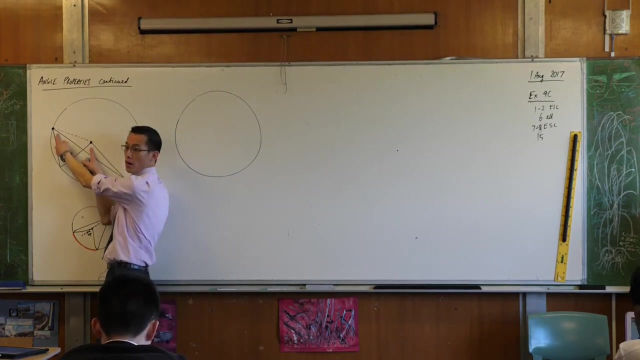 and I'm going to join it up to the center like so, Excuse me, So how am I going to get to? like, what's my aim? I want to show that this angle in here is double this angle over here, okay, And I want to use some basic geometry and 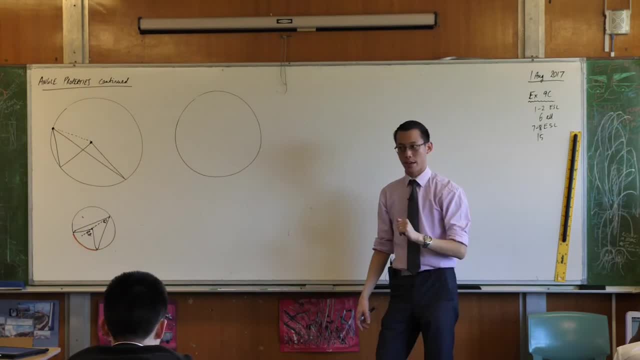 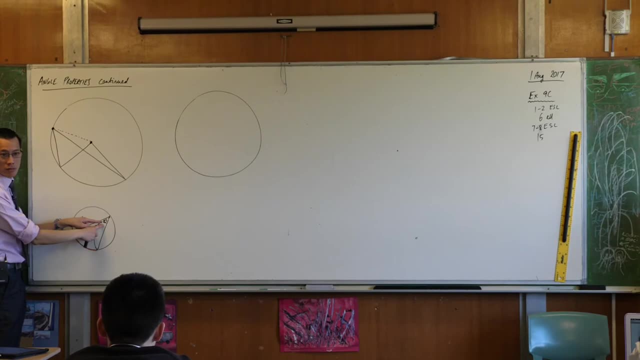 I saw these triangles because we know they're everywhere. to prove that, Let's begin by just giving some names to these things, okay? So do you remember what I called? I called each of these little angles that make up the angle of the circumference. I called them. 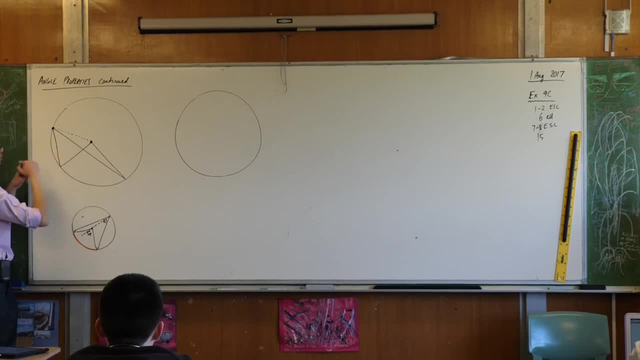 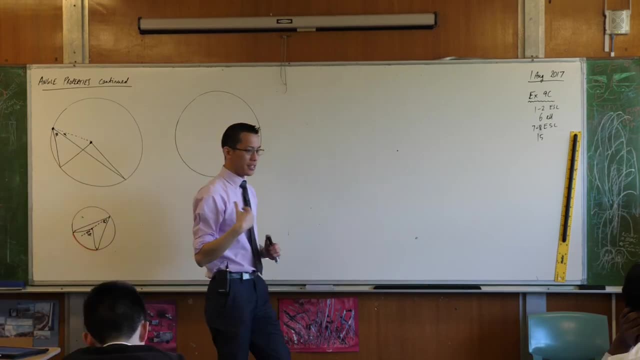 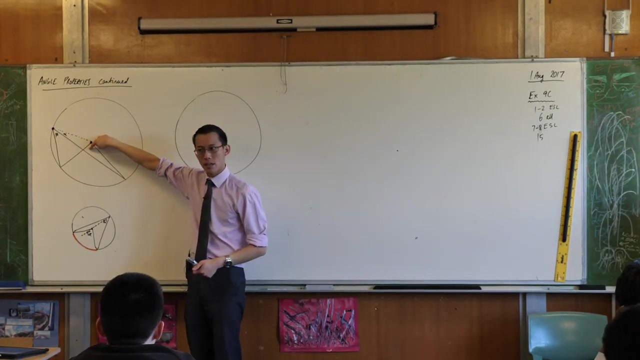 any names, I like I think I called them alpha and beta. do you remember that? So I'm going to call this guy alpha and this guy beta. okay, The difference here is that the angle I'm going to end up with this one in here it's not going to be 2 alpha plus 2 beta, is it In this case? on this diagram, what do I want that angle to be? 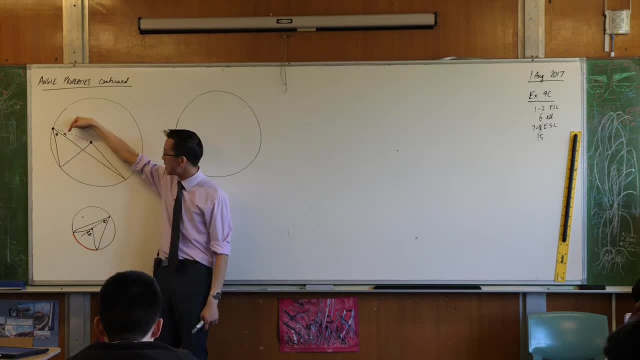 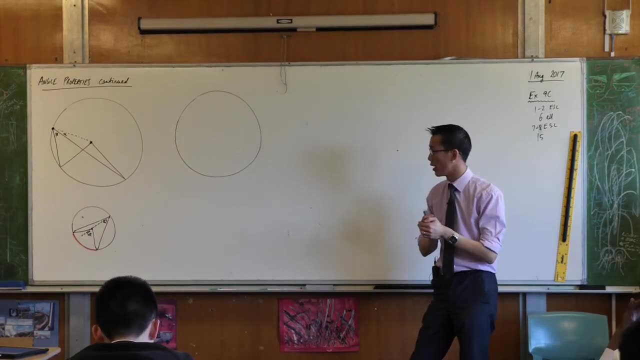 Just 2 beta, just double that angle on the circumference. The alpha is not included, but it's kind of hanging out there on the side. Okay, there's loads of isosceles triangles in here. I can see at least two that relate immediately to the two angles that I've just drawn. 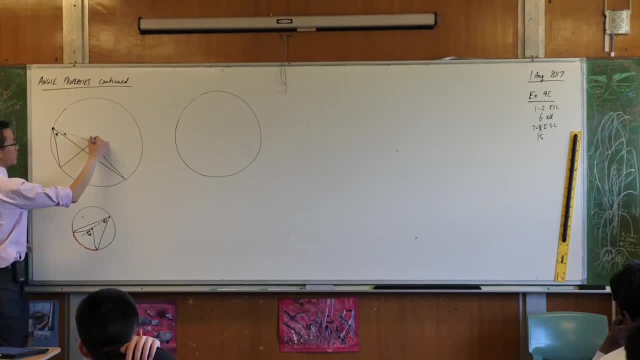 Anyone want to suggest to me? let's put some names on this, shall we? Let's call this O. let's call this A, B, we'll make this guy C. Would anyone like to describe an isosceles triangle? oh, I should name this. let's call that P. Would anyone like to describe an? 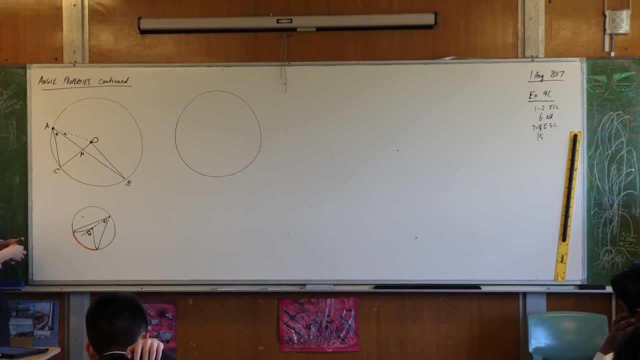 isosceles triangle for me and tell me what to put in there. AO, OB- these guys are radii, Let's mark that in. So therefore, what statement can I make about angles that goes with that pair of equal signs? Any takers? Everything is named. you don't have. 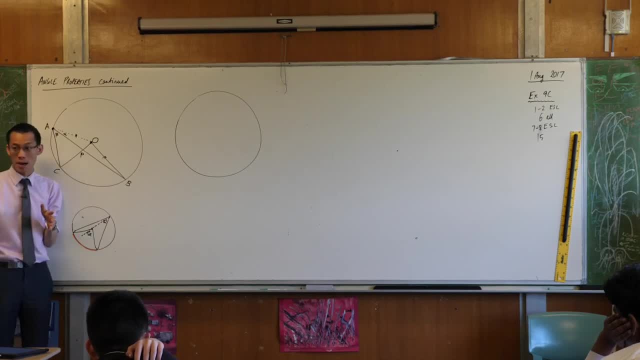 to point. you don't have to use vague words. you can tell me which angle you mean. yeah, O B P is equal to O A P. Thumbs up right. Those are both the. they're the base angles of. 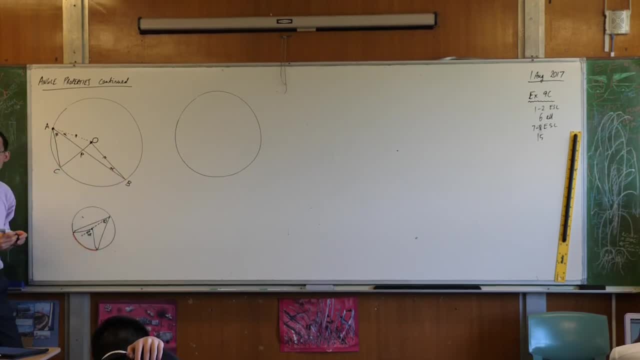 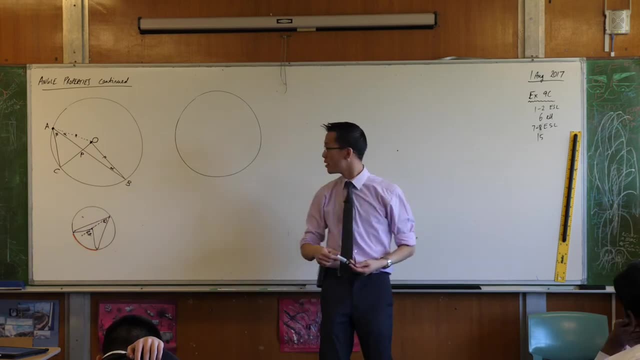 this isosceles triangle right, So that makes that alpha Okay. so far, so good. There's another isosceles triangle in there. can you tell me where it is? O, A and O C, also radii, So in fact. 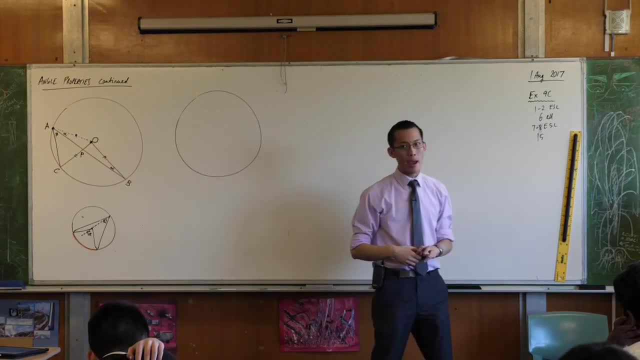 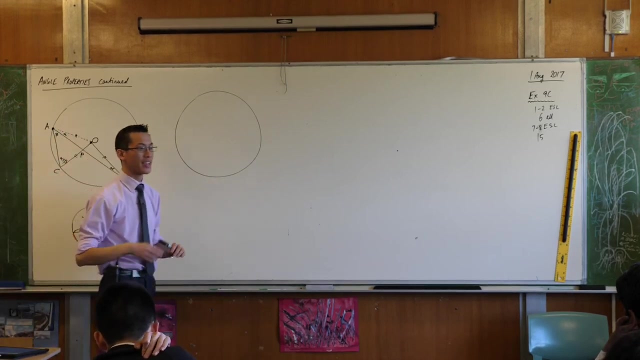 I can mark in that as equal. So what would be the pair of equal angles that matches that pair of equal signs? Okay, so you've got alpha plus beta in this corner, which means you get alpha plus beta in this corner. So far, so good. Are you happy with that? Me too. Okay, now pause for a minute. Here is 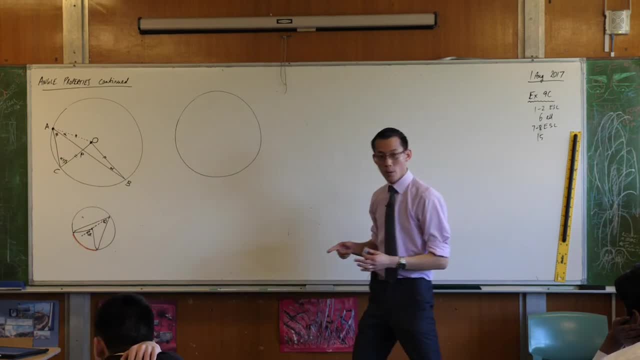 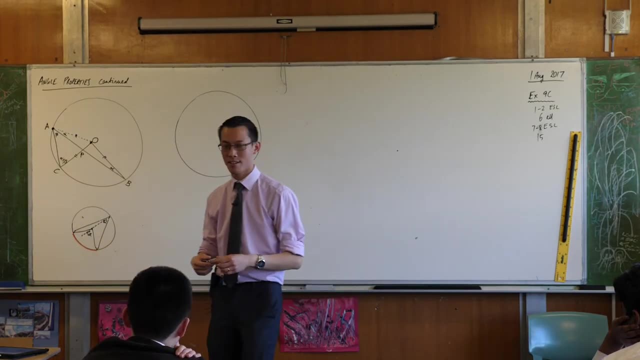 the interesting part. We've done the easy bits. Remember where I want to get to. I want to get to here. Let me give you a couple of minutes to have a think about how you'll get there, if this is easy. So if you've got an idea, call me over Done. What I would like today is make sure your 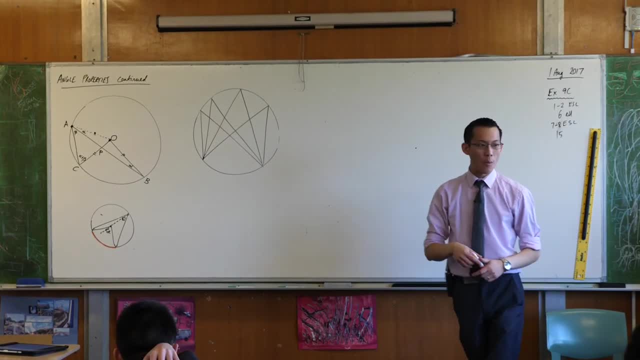 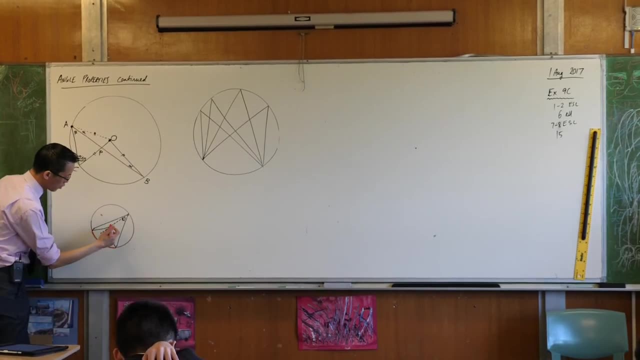 pens are down, your eyes are up because if you blink you will miss it. It's that quick, okay, I want you to look at what's there and I also want you to remember how we did it last time. Do you remember, for instance, if I called this alpha, then you got another alpha in the corner?